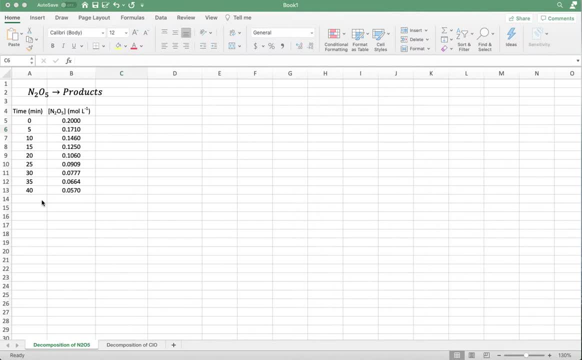 concentration of the reactant decreases, And so what we want to do is plot this data and use that plot to determine the order of a reaction based on experimental data. In the first example, we're going to plot this data and use that plot to determine the order of the reaction. Now, when we plot the time versus, 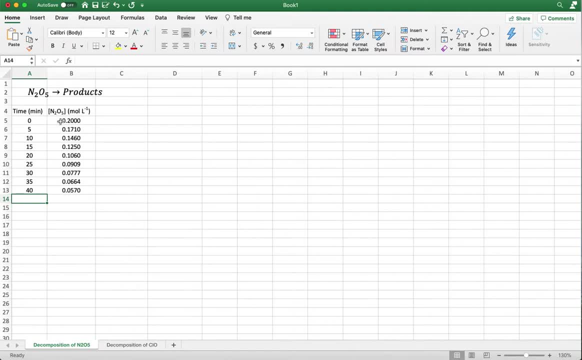 concentration data. remember, if we get a straight line, we have a zero-order reaction. So let me show you how to make these plots. in Excel You'll plot the time on the left-hand side, the concentration on the right-hand side. In Excel you can go ahead and highlight the time on the left-hand side and 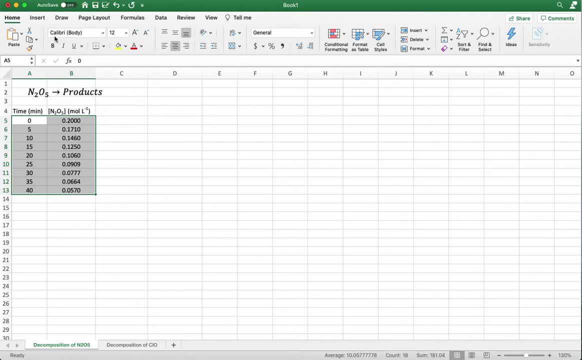 highlight both of these columns, Click Insert And, based on your version of Excel, this may look a little different, but generally in Insert you'll have the charts somewhere in here And we're going to use what's called the XY scatter. And of course it's called XY scatter because the time on 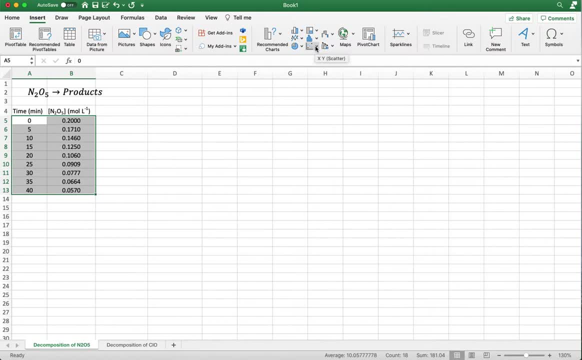 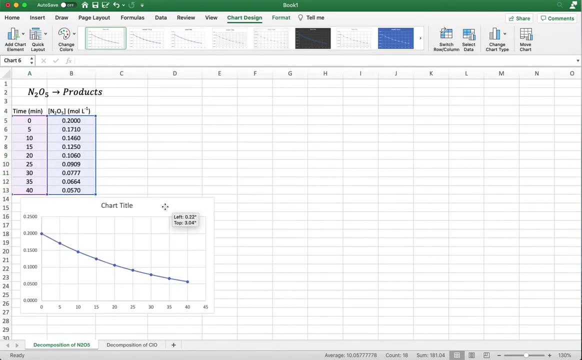 the left-hand side, that's your x-axis and your y on the right-hand side will be your y-axis. So I'll click this And if you click the arrow, you'll be given different options of what to plot. So I'll go ahead and plot the line with the dots And, of course, here you go. So this is. 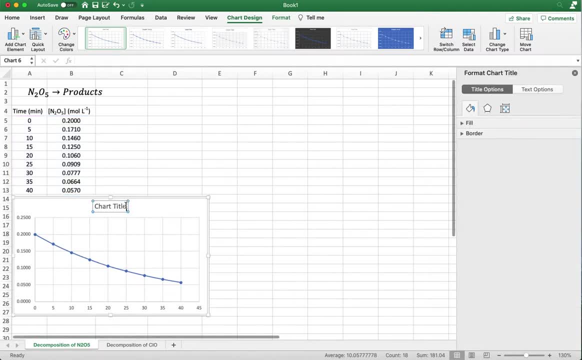 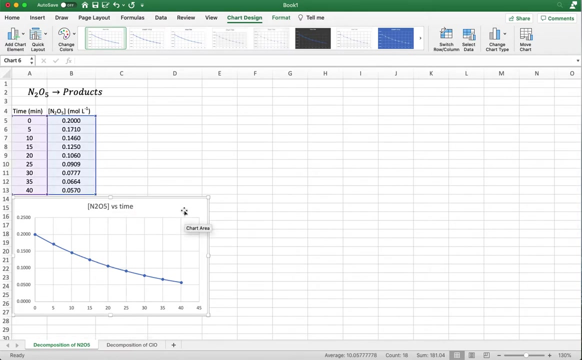 what that looks like, And I'll rename this title as N205, in brackets, for concentration versus time. So this is the test for zero-order reactions. And remember, if we plot the concentration versus time, if we get a straight line, then that means this is a zero-order reaction. Now you can see clearly. 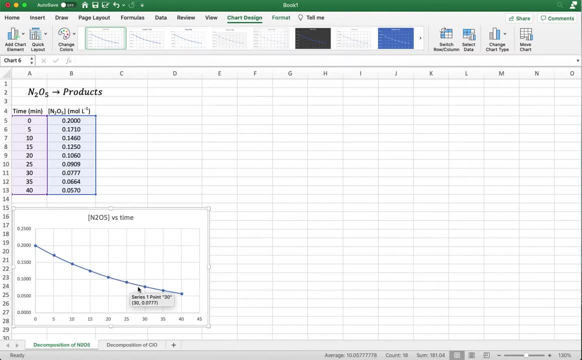 this is not a straight line. There's a kind of a curvature here. as we go right around 20 minutes, 25 minutes, it starts curving. We can insert a line just so that this can you can visualize it a little bit better And so you can see the red line right. 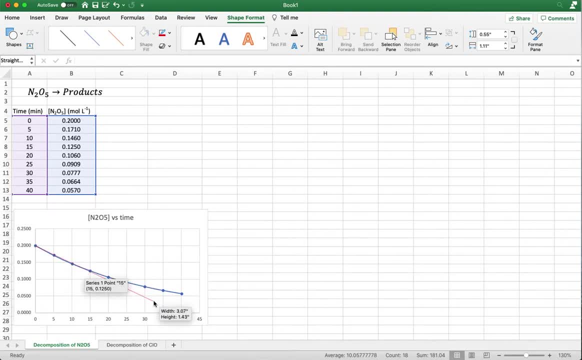 If I kind of connect those dots, you can see clearly that this is not a straight line. So there's a curve there. So what does that tell us? This tells us that this reaction is not zero-order. So what we'll do is we'll test for first-order. So let me make a note here. 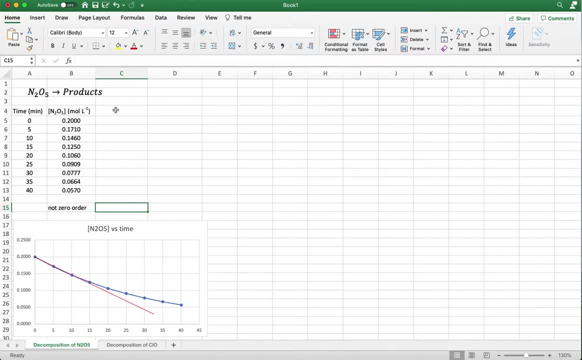 So what we'll do next is test for the first-order reaction, And so one column over. remember, when we test for first-order, we're going to plot the Ln of the concentration of N2O5 versus time, So one column over. that's where I'm going to get my data. Now. Excel, if you're not familiar with it, can do these calculations for you. 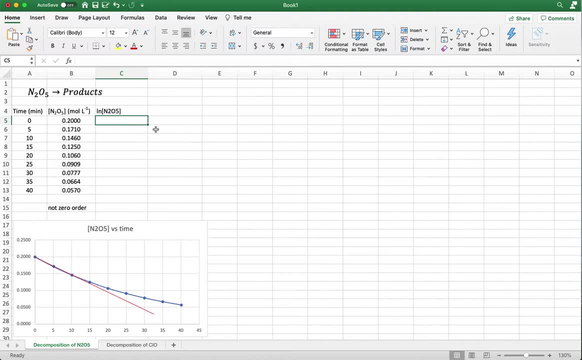 very quickly. So let me show you how to do that. Instead of going one by one with your calculator and finding the natural log of the concentration, what we'll do is we'll use Excel to do that for us. so in that cell at time equals zero minutes. we'll go ahead and put equal sign. 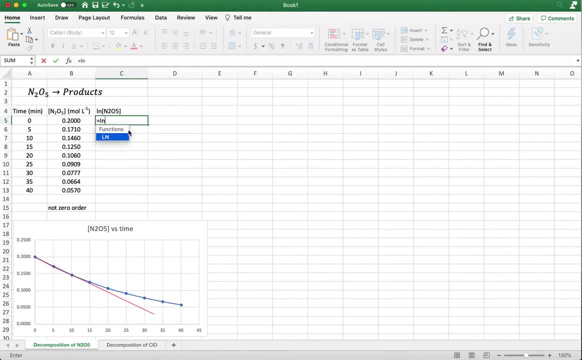 we'll type in the letters ln and you see that the function comes out for the natural log. we'll put a parenthesis and excel is telling you that there's a number that goes in the parentheses. but in this case what we'll do is we'll click this cell, because this is what we. 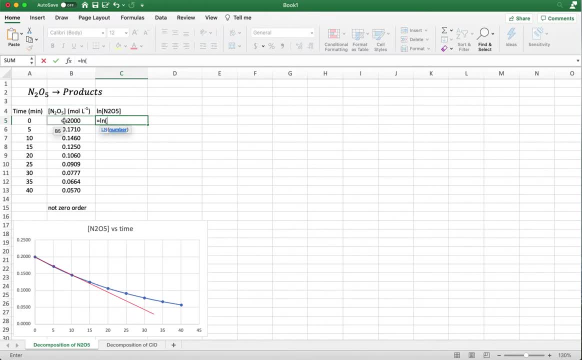 want the natural log of the concentration. so 0.2 is this first concentration. so that's cell b5 and close parentheses. and that's your equation. that's your calculator. press enter and there you go. so there's your natural log of the concentration. now we've got to do that for each one of these, but of course excel can do that for us. you see that. 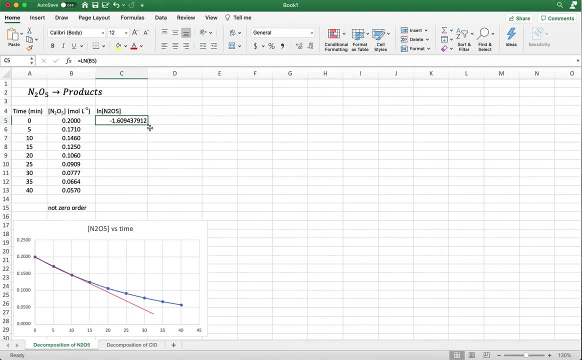 green box on the bottom right hand corner. you can hover over that box. you see that black cross, click and hold, drag down, and so you can see that from the function box. you can see that. you see that we kind of go down for each um concentration and there you go. 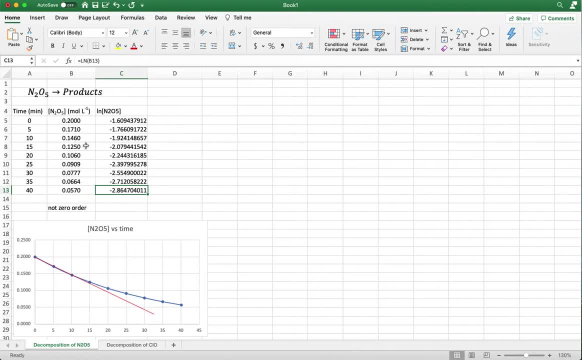 okay, so let's go ahead and plot this and let's check our graph. so again, we're going to highlight the time, but now we got to skip over to the natural log column. now to highlight just the natural log column. i want to make sure that i'm not missing anything here. 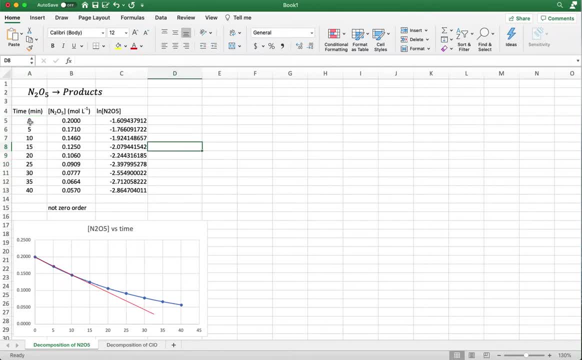 i want to skip the middle column right, so you can't just click and hold, because everything will be highlighted. so we're going to have to select this and if you don't know how to do that, i'll show you. highlight the time column and go ahead and click control. if you're on a pc, if you're on a 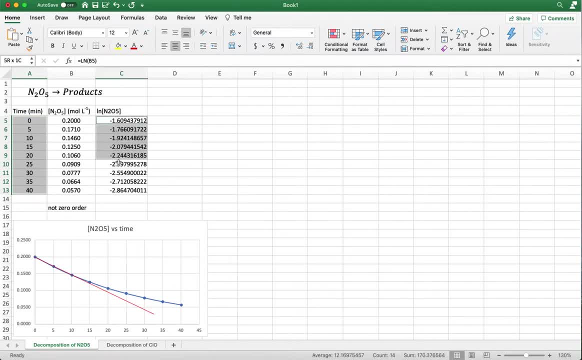 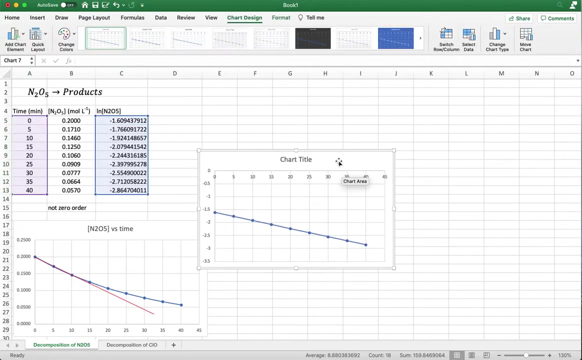 mac, you can click command and highlight the other column and you see that the middle column is skipped, which is what i want. i don't want that data. so now i have column a and column c and, just like we did before, insert, go to our graphs and i'll graph the x, y scatter with line and dots, and here's our plot. 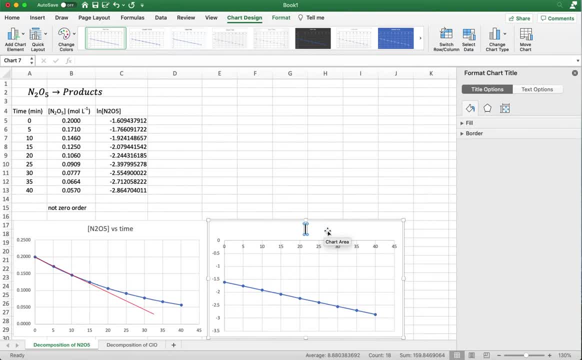 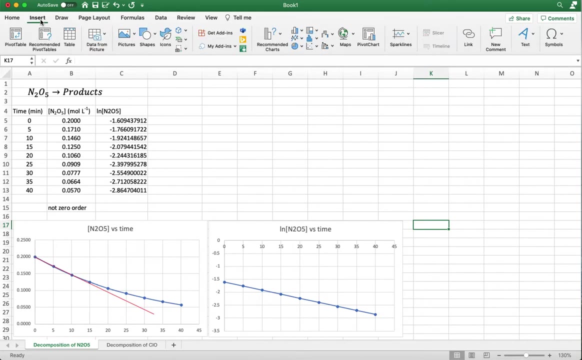 and i'll go ahead and rename that the natural log of n205 versus time. so here i'll insert a line, just so we can check this. this looks like a pretty straight line, and so i'll go ahead and color this red and if i just connect the dots, the first two dots, you can see this. this lines up really well this. 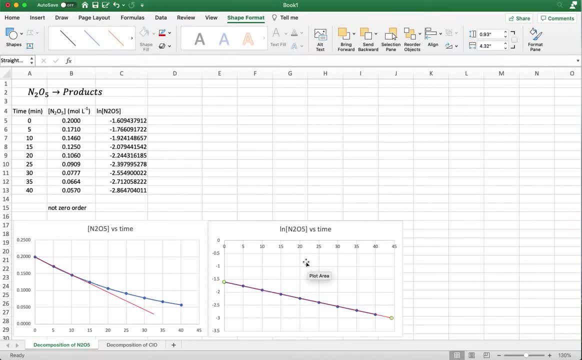 is a really nice straight line and so it's looking a little, uh, a lot like. this reaction is first order kinetics. in other words, this reaction is going to be n2, or the rate law would be rate constant times, n205 raised to the one, and we determine that from the graph. 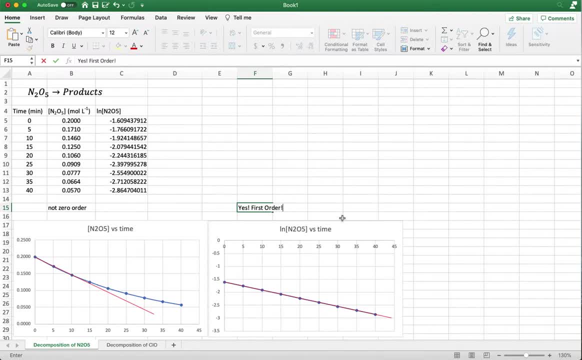 okay, now, just for good measure, we'll go ahead and just plot the test for the second order, just so that we can see what it looks like. now again, if we're going to plot the test for the second order reaction, we're going to plot 1 over the concentration of n2 o5. 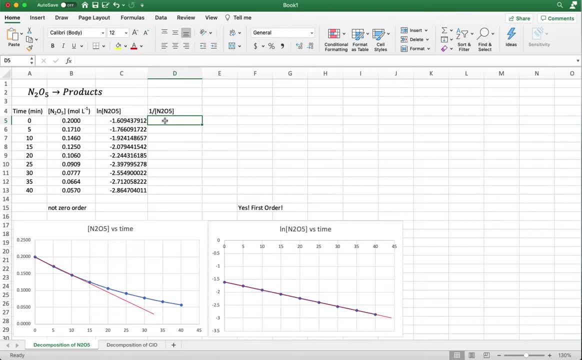 versus time. so we need the data, we need this number here for the inverse of the concentration. so again we can have our calculator in excel do that for us. so we'll press equal, sign, 1, slash or divided by. now there's no function here. i'm just going to click the cell b5 and so. 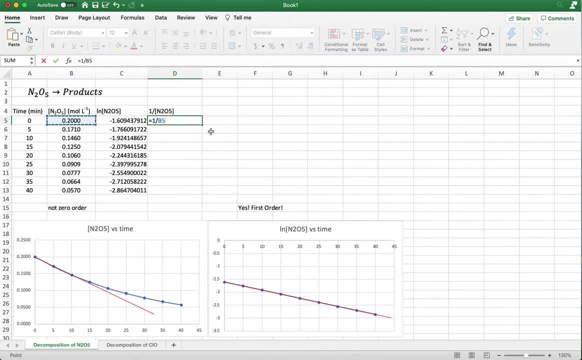 my calculation is just 1 over b5 and press enter, and so the inverse of 0.2 is 5. and we need to get the inverse for all the other concentrations. but of course here's another little trick for excel: you can hover over that bottom right hand corner. 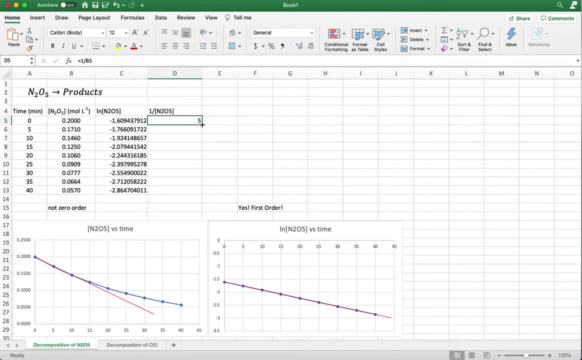 that green box, when you get the black cross, you can click and drag, just like we did before, or you can actually just double click and it'll go down the column and give you that data. so again, we'll go ahead and just plot the time versus the inverse of the concentration. so again, if you're on a pc you can control. 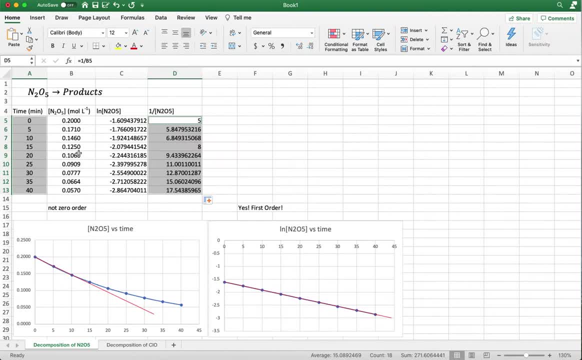 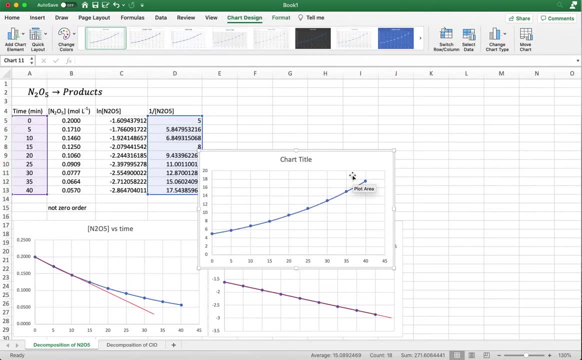 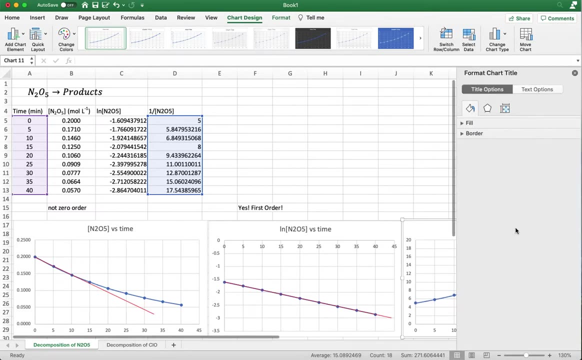 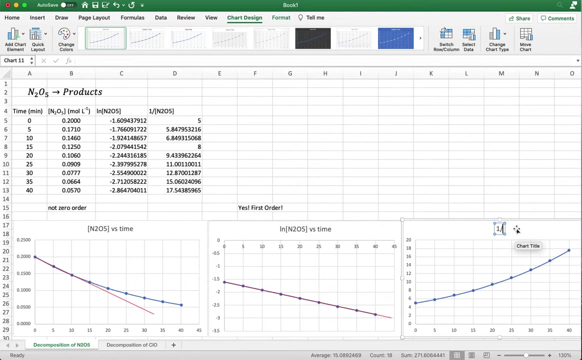 if you're on a mac, you can press command and hold that and you highlight those two columns and we'll insert our xy scatter and okay. so really nice graph here. you can see that there is again just another curvature or curve line, and so we'll rename this as one over and two oh five. 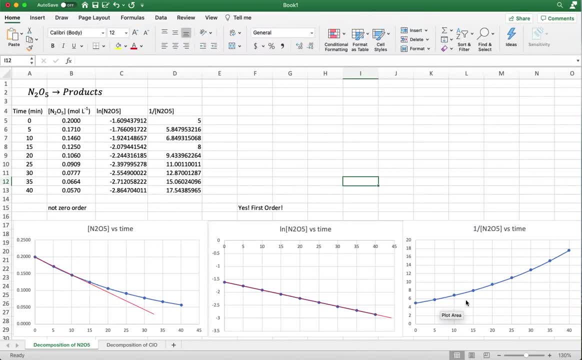 versus time, so clearly there's a curve there. i'll go ahead and insert a line again just so we can see it a little bit better, and we'll highlight that in red. and so if i connect those first couple of dots right, clearly you can see that this does not stay in a straight line. it actually curves. 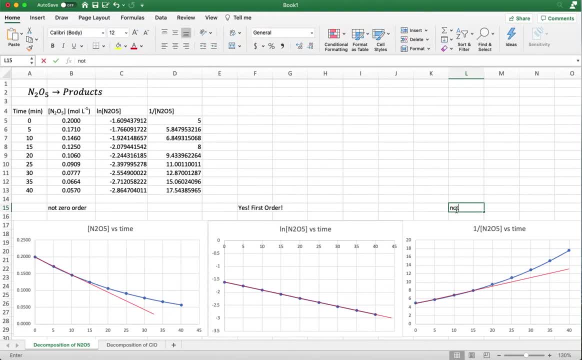 so this is not a second order reaction. okay, so what we've done here is shown you how to plot in excel. plot the experimental data in excel and we can plot different graphs. we can actually calculate the natural logs and the inverses of the concentrations so that we can test for first order and second order reactions. 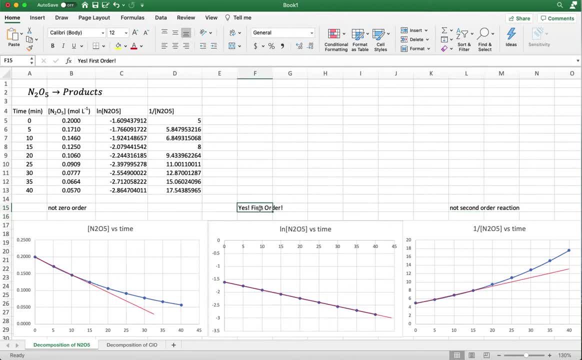 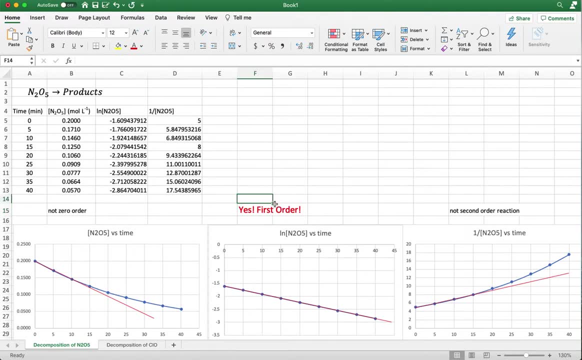 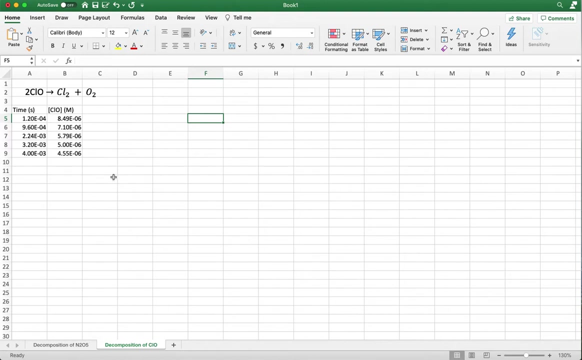 so in this particular example, this is a first order reaction. let's do one more, and so i have another example for the decomposition of c l o. so again, we want to test for zero order, first order and second order. so i have some data here, i have time in seconds and i have concentration in molarity or mol per liter. 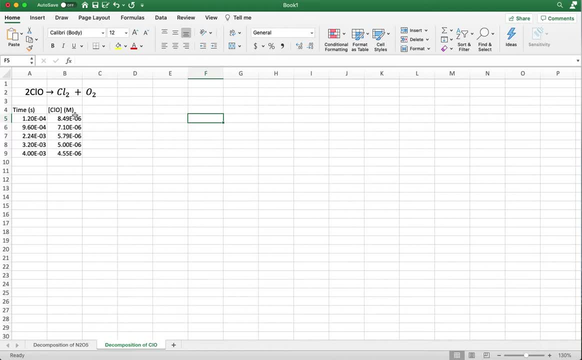 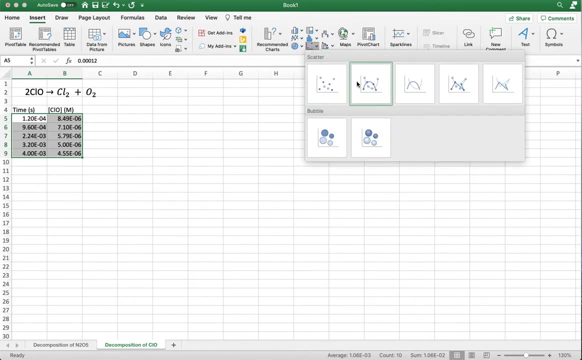 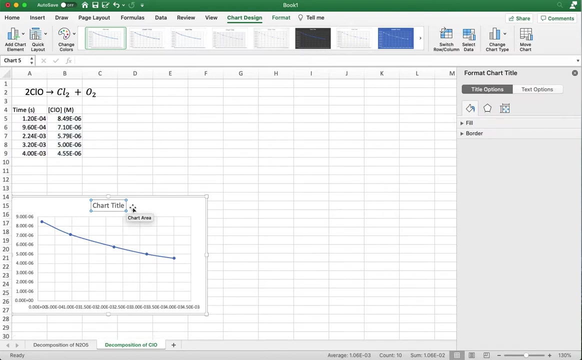 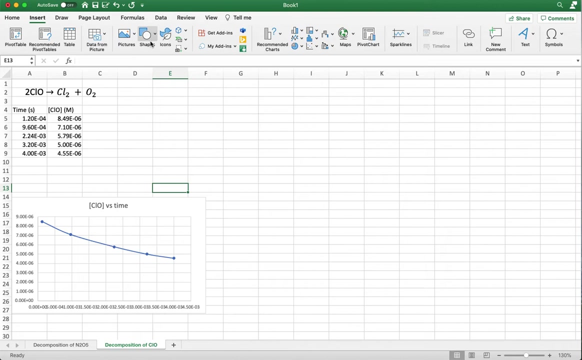 now remember, for kinetics we can also track the partial pressures if we're dealing with gases or if we have data for gases. so i'll go ahead and plot the concentration versus time, insert the xy scatter and this graph does look like it's a curve again. i'll go ahead and add a line just so we can. 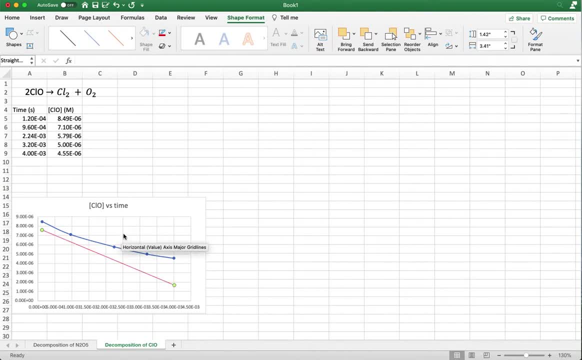 see it a little bit better and i'll color that red. and so again, just plain, connect the dots here. you can clearly see that this is not a straight line. so again, not zero order. so we need to continue our tests now. let's test for first order reaction and we'll. 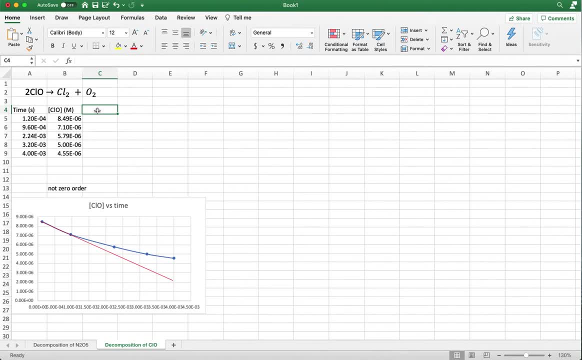 have to plot the natural log of the concentration versus time. so in the next column over i'll type ln, bracket c, l, o, close bracket, and i need to get my data for the natural log of the concentration so that i can plot the natural log concentration versus time. So just like in our last example, 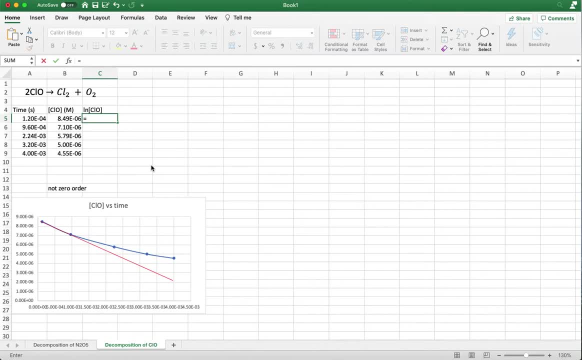 we'll press equal natural log ln, Because the natural log is a function you do have to put in the parentheses. So open parentheses, highlight your cell, and close the parentheses, And so we'll get the natural log for the cell B5.. There we go, Bottom right-hand corner of that cell. we 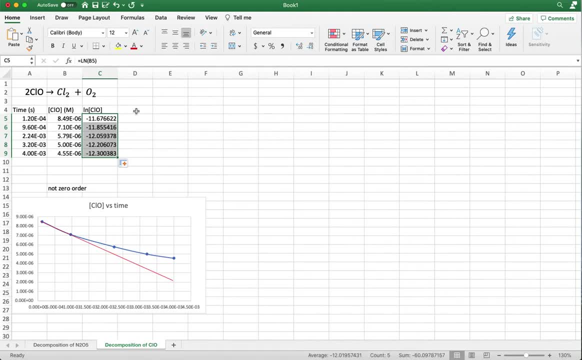 can double click and that'll get us the natural log all the way through. And as long as I'm here, I'll go ahead and plot or get the data for the inverse, And so we'll click enter. I'm sorry, equals. 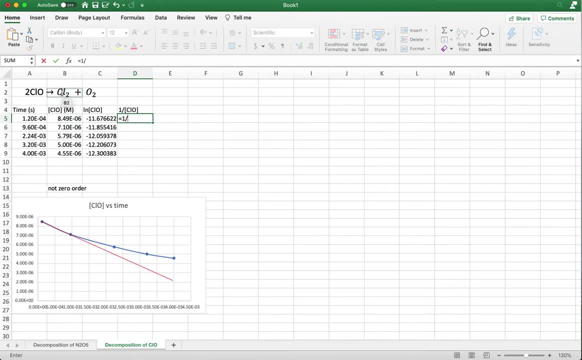 One divided by, and again go back to the original concentration and double click the bottom corner And here's our data. Okay, so let's go ahead and get our graphs and then we'll study them. So here's the time versus the natural log. 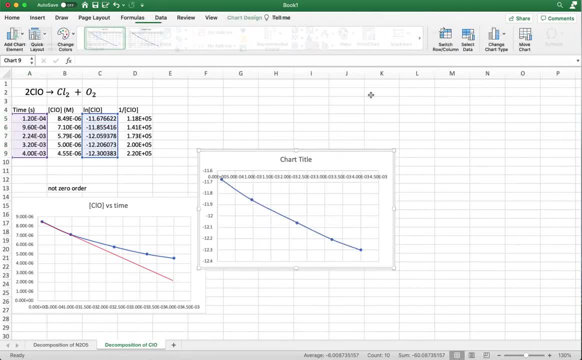 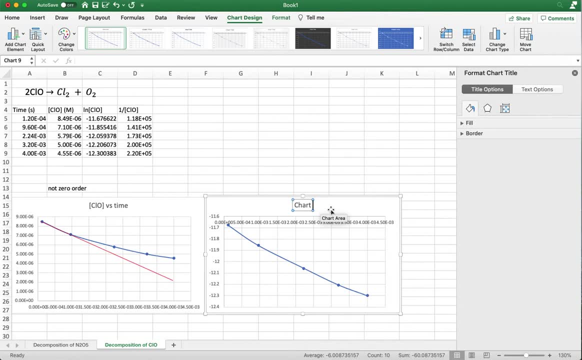 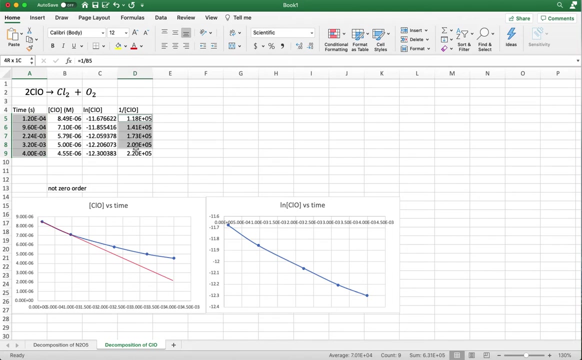 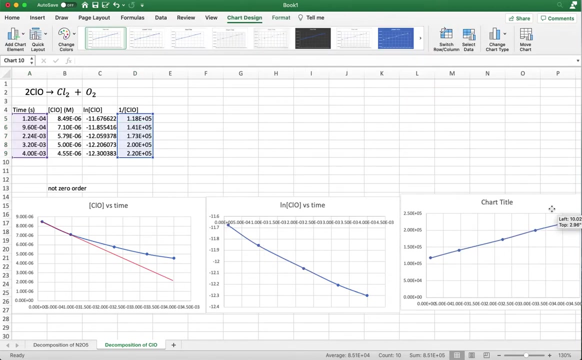 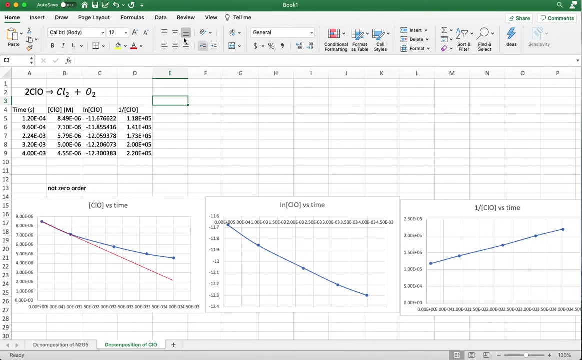 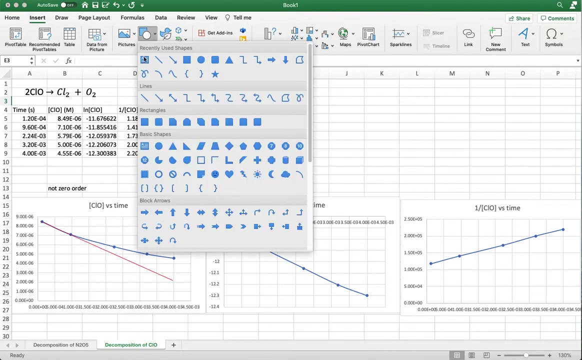 Insert our chart. That looks a little curvy. Let's check the inverse and insert, And that does look pretty straight. That looks pretty straight. Okay, So this is the test for first order and second order. It looks like this is going to be a second order. whoops, a second order equation, or?